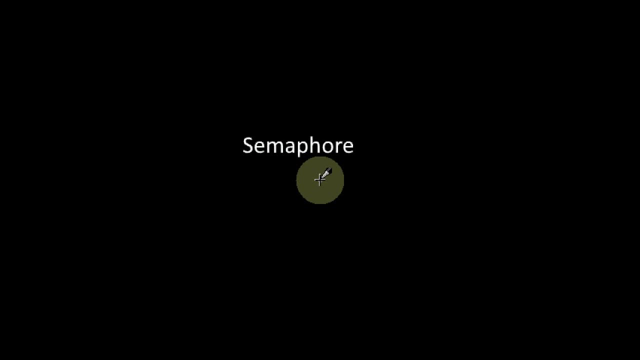 These are solutions to just the critical section problem and the process. synchronization is not just about the mutual exclusion and critical section problem, Sometimes ordering the execution of the processes and the management of resources, everything may be required. The previous solutions we discussed cannot be extended for other synchronization issues. 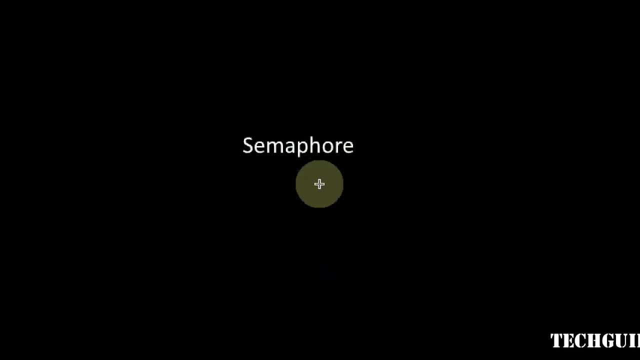 But semaphore is possible. It is a synchronization mechanism that can be used not only for critical section problem, but also for other synchronization issues. Now, what is a semaphore? Semaphore is just an integer variable. We can name it as S, or if we are using it for solving mutual exclusion, then we can name it as mutex mutual exclusion. 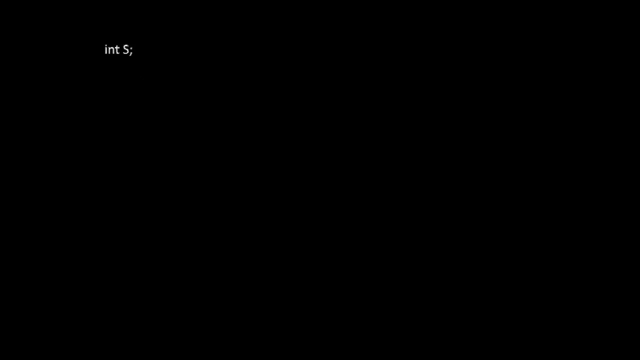 Then there are two functions associated with this semaphore variable. One is weight of S and other is signal of S. Otherwise, we can name it as P of S and V of S, or down of S and up of S. Now what the user should do is depending upon the synchronization issue we have to solve. 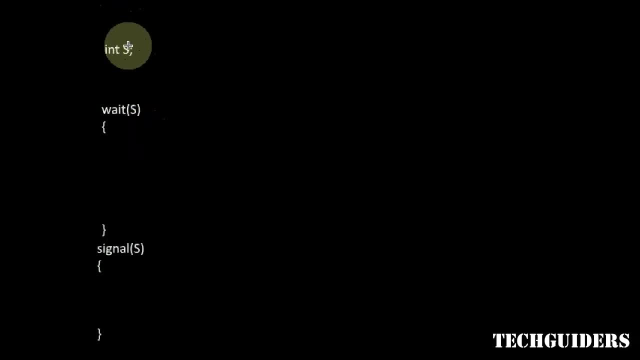 we should initialize the semaphore variable with a particular value And after initialization we can access this variable only using these two functions. We cannot access this variable directly. So the value with which this variable is initialized depends upon the synchronization issue we have to resolve. 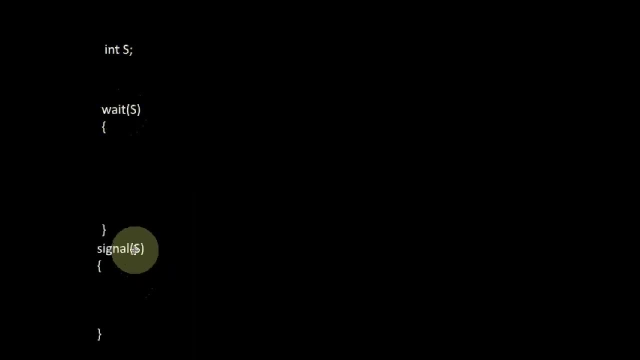 Also how these functions work. So the value with which this variable is initialized depends upon the synchronization issue we have to resolve. Also, after initialization, we can access this variable only using these two functions. Also how these values work. So the value with which this variable is initialized depends upon the synchronization issue we have to resolve. 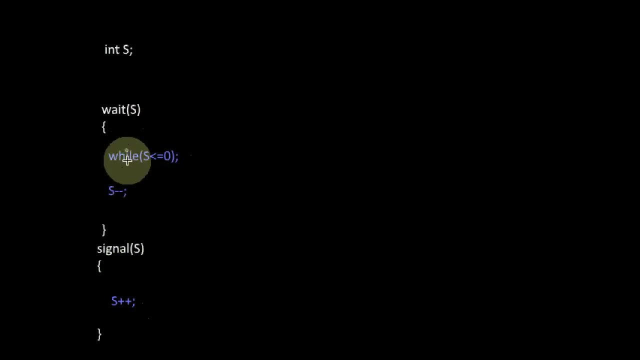 And these are the classical definitions of the functions. The Waite function is a decrement function and this function waits for something, waits for a result or waits for a chance to enter. the critical section based on the value of this semaphore variable is, if the value of the semaphore variable is not greater than zero, then the process will wait in.